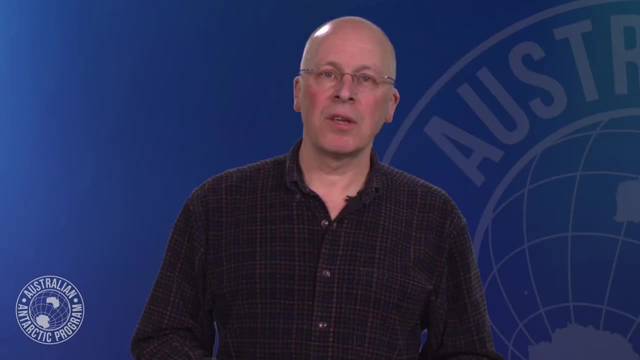 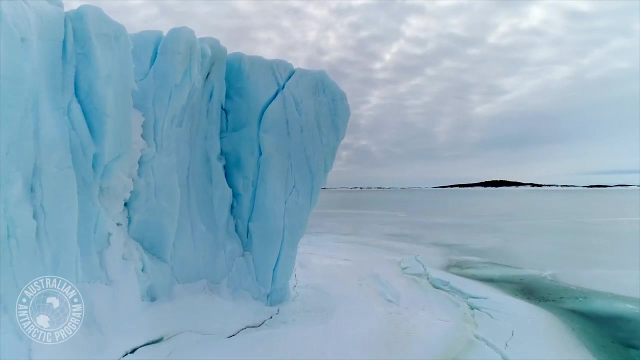 want to talk about here is why we were doing what we're doing. that's an interesting question. I mean, Antarctica is a fantastic place, privileged to work there. it's stunningly beautiful, harsh and captivating, but that's not the reason why we're there. you see, Antarctica matters in very direct. 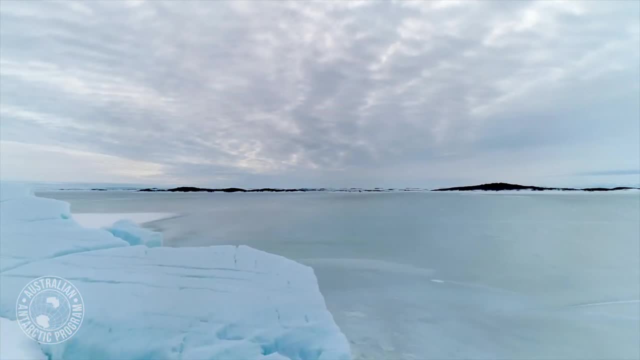 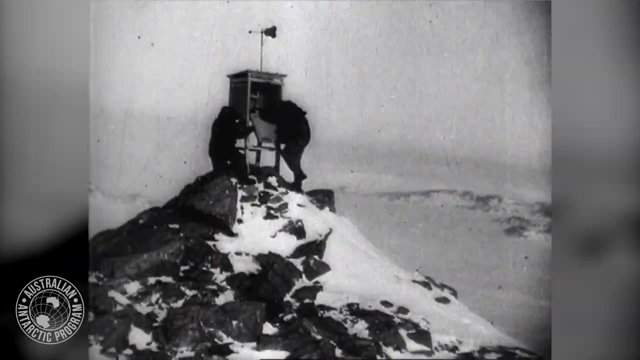 ways to all of us. The early explorers Mawson and colleagues understood some of this. they knew that Antarctica was important for the weather of Australia and other southern hemisphere continents. in the 100 years or so since, we've learned a great deal more and we know now that Antarctica 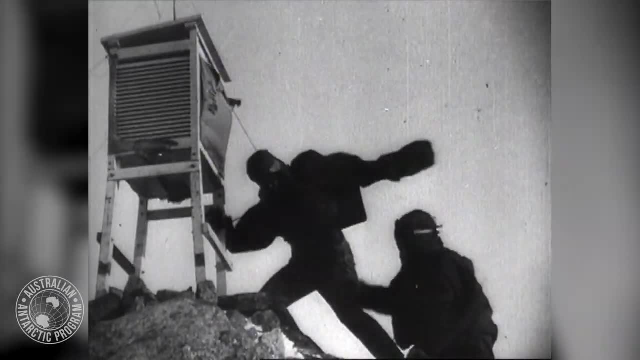 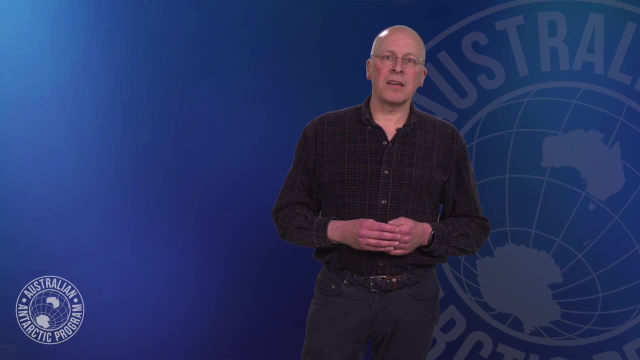 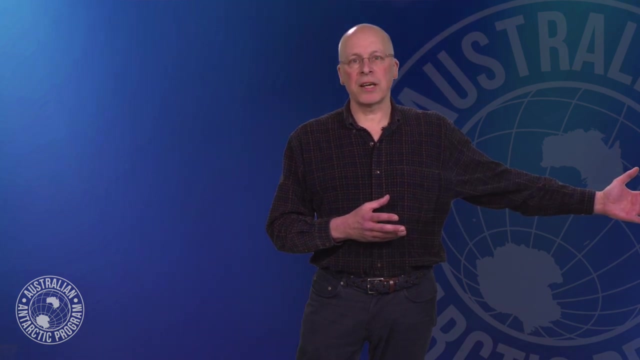 and the southern ocean are engine rooms of the global climate system. I'm a glaciologist and a climate scientist and I work in a team of scientists here who are studying the how Antarctica fits into the global climate system. We look back at the climate past from ice cores and other sources of evidence. we look at how things. 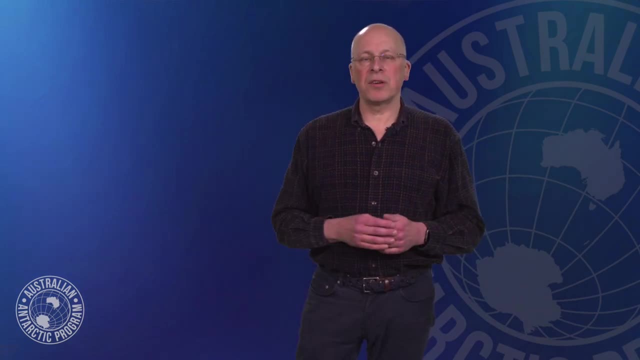 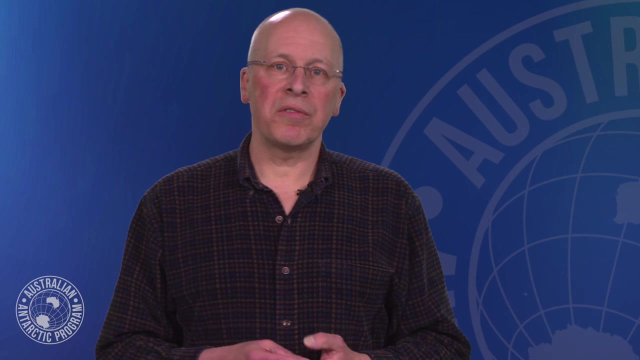 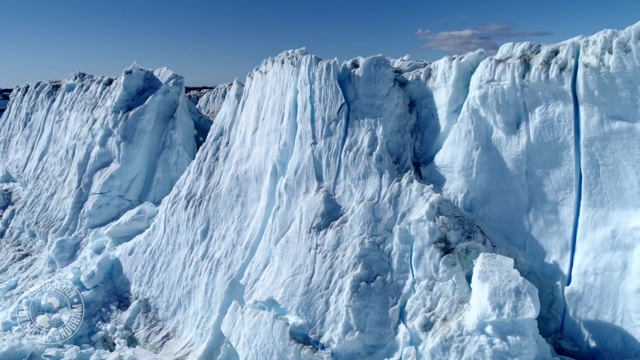 are now and how they're changing, all so that we can better predict where we're headed in the future. What I want to do now is just take you through some of the areas of study and give you a feel for what that work involves. When we think of Antarctica, of course, we think of ice. it has more than 90 percent of the planet's. 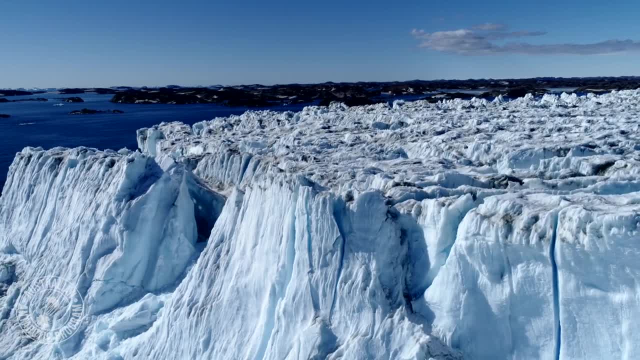 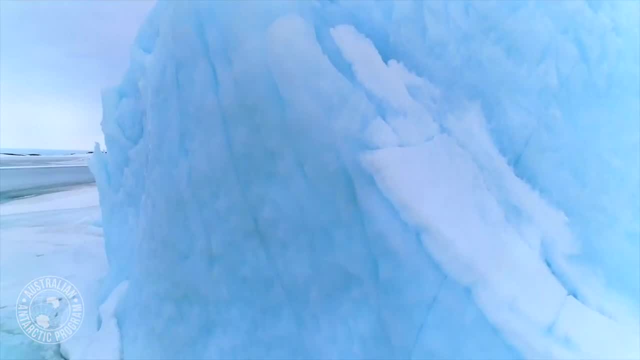 ice and in fact, if it was all to melt, it would raise sea levels by 60 odd meters. We know that in the past, Antarctica has had ice sheets for tens of millions of years, but we do know from the past that the waxing and waning of the Antarctic ice sheet influences sea. 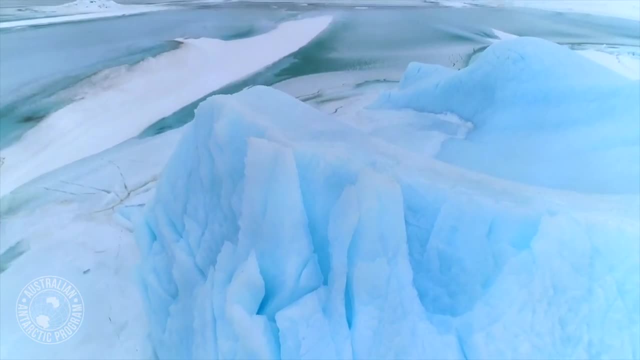 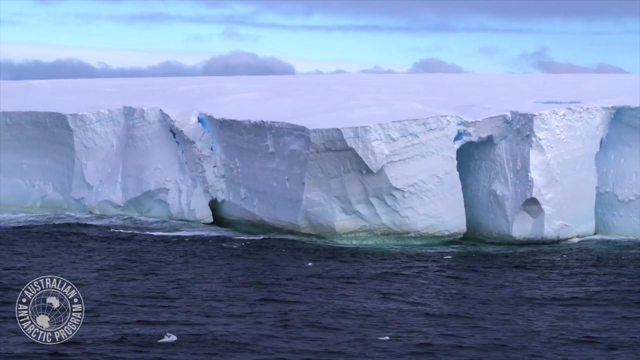 level. Last time temperatures were two to three degrees above pre-industrial. roughly where we're heading if we overshoot the Paris targets. Sea levels were six to nine meters above present. How that plays out in our warming world. what's the timing, what are the rates of change? where? 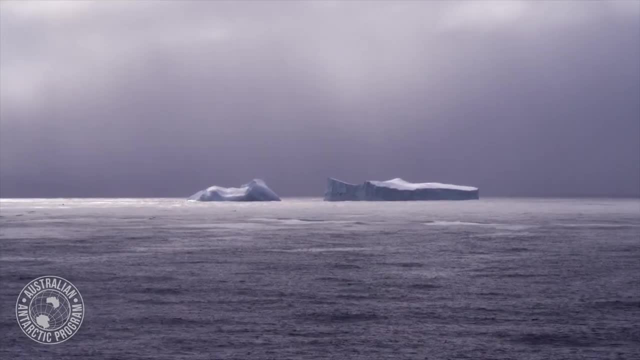 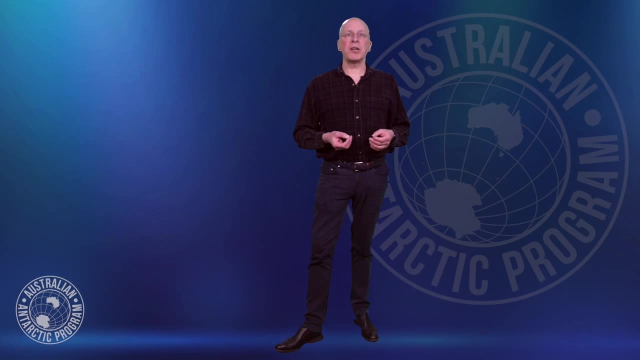 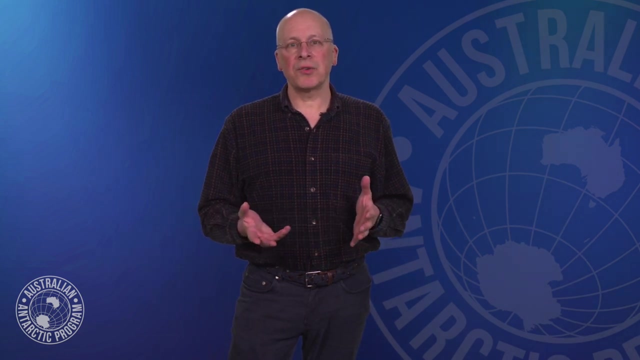 are? the vulnerabilities are key questions for Antarctic glaciologists. The best we can say at present is that sea level rise by the end of this century- 2100, will be between about 29 centimeters- if we mitigate really hard- and 1.1 meters. That's a distressingly large. 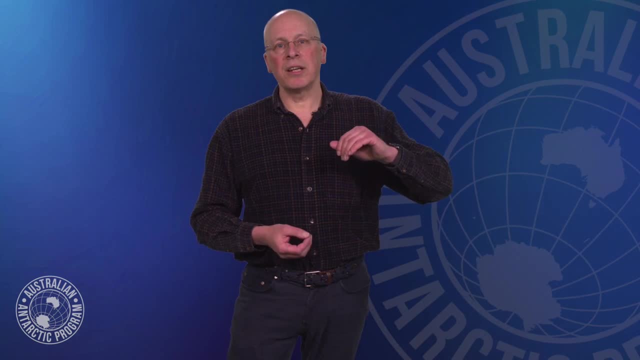 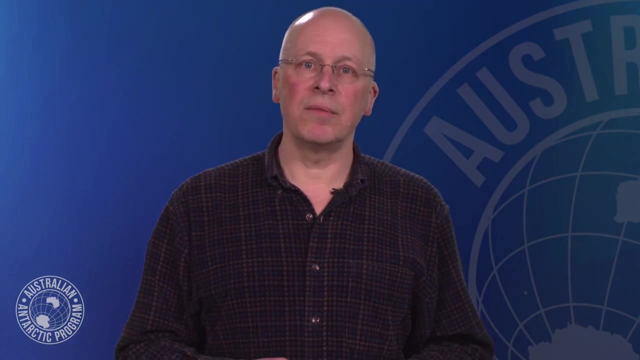 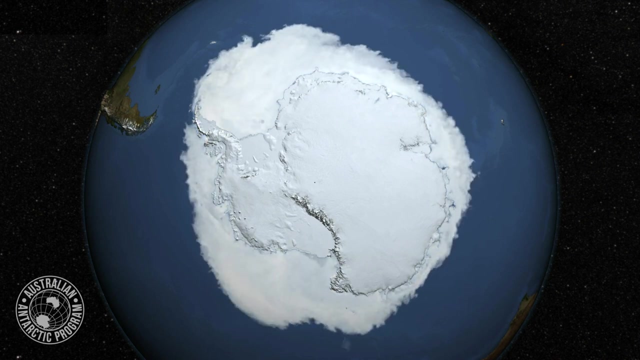 range, and it overlooks the fact that that's only the likely range. The actual sea level rise could even be higher still, and of course, we care what happens beyond the year 2100.. Ice is also a feature on the oceans around Antarctica. Every winter we see a growth of the sea ice around Antarctica, the frozen skin. 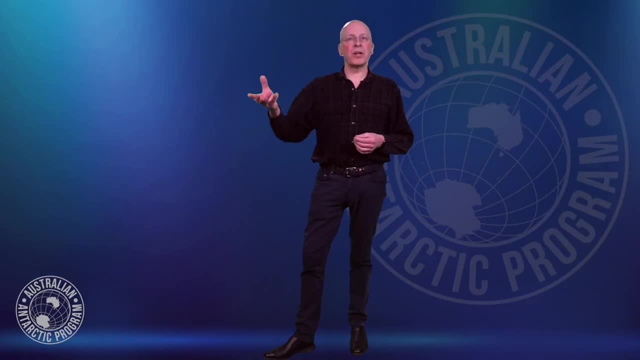 of ocean, on average around a meter or so thick, more in some places and less in others. The sea ice plays a critical role in the climate system by reflecting light back to space and actually regulating the flow of heat and moisture between the ocean and the atmosphere. 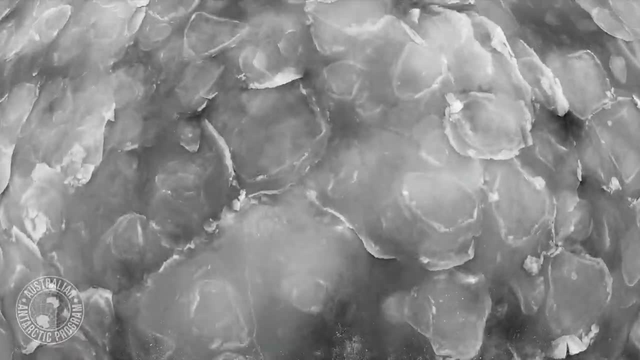 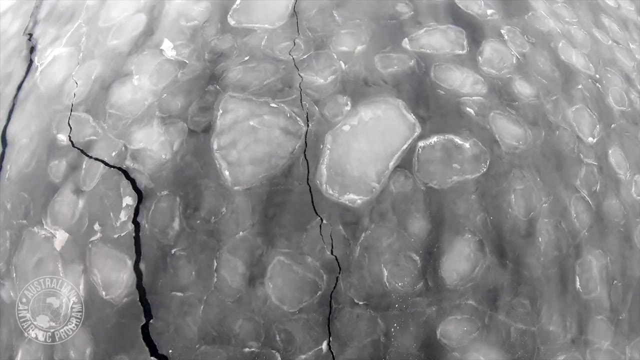 Sea ice is also really important for the Antarctic ecosystem, but that's a separate story. When we look at how sea ice has changed over recent decades, we see that in the Antarctic, if anything, it's increased very slightly, unlike the Arctic, where sea ice has gone down. 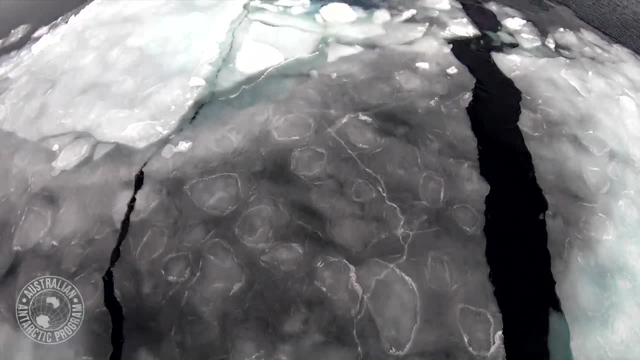 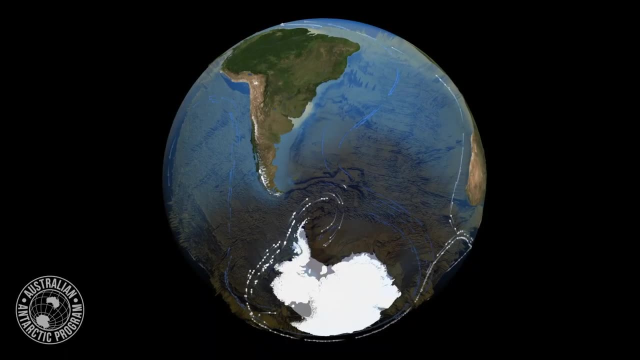 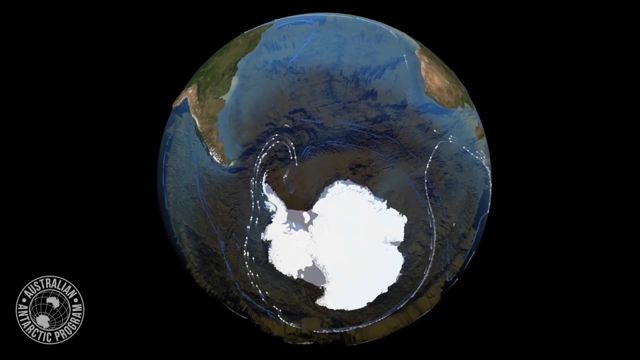 precipitously, Although in the last few years in the Antarctic we've also seen a reversal and a starting of a decline in sea ice. We understand parts of what we're seeing here. We understand the importance of ocean currents and winds and the input of fresh water from the ice. 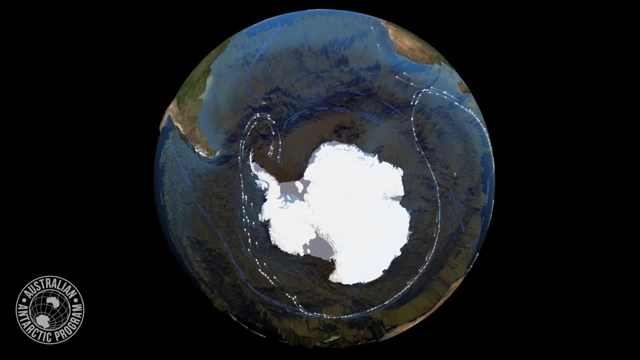 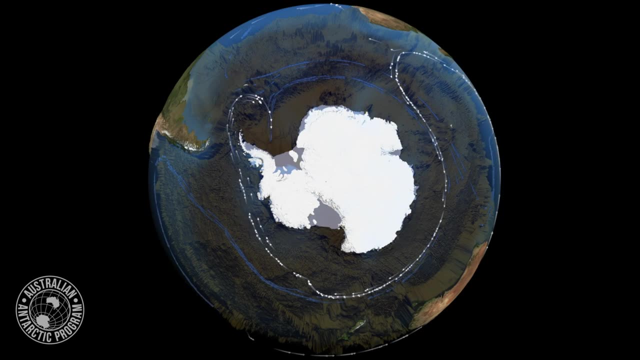 sheet and from precipitation. All of these jigsaw pieces are important, but we don't have the overall picture of where sea ice is heading, how fast is it going to change and what does that mean? The ocean around Antarctica is also important. It connects Antarctica to the rest of the planet. 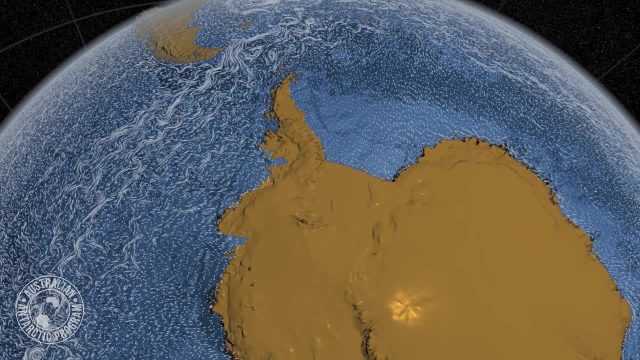 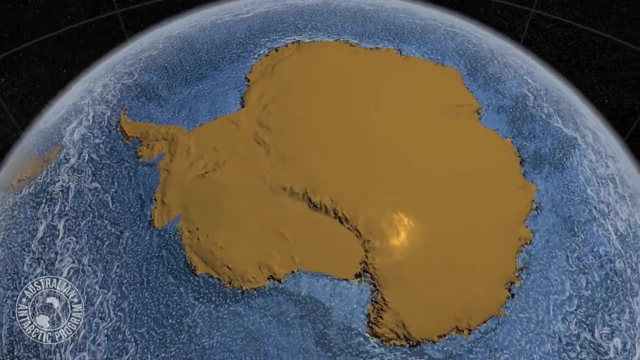 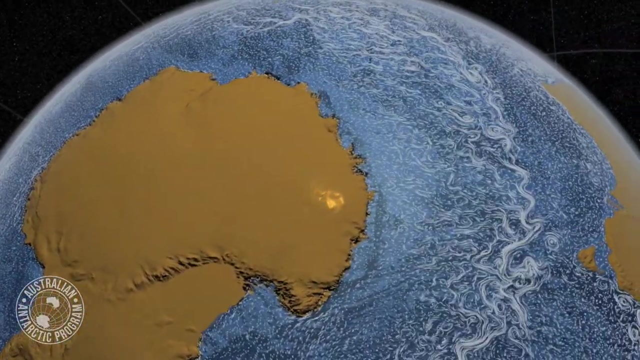 through deep ocean currents that travel around the globe. The largest of these currents is the Antarctic Circumpolar Current, which, as the name suggests, travels all the way around Antarctica, connecting all of the ocean basins. It also actually regulates the mixing of deep ocean water and surface waters and, along with the 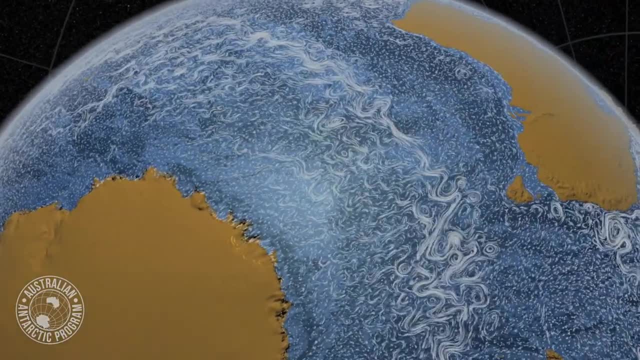 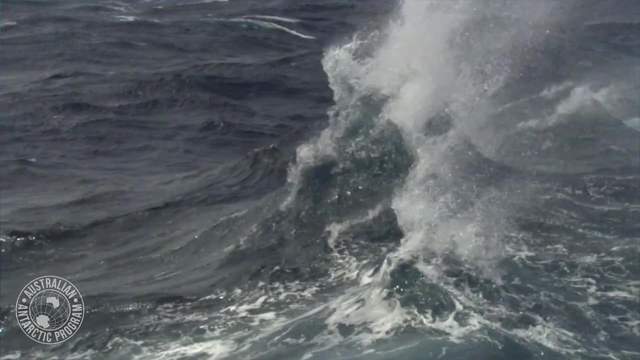 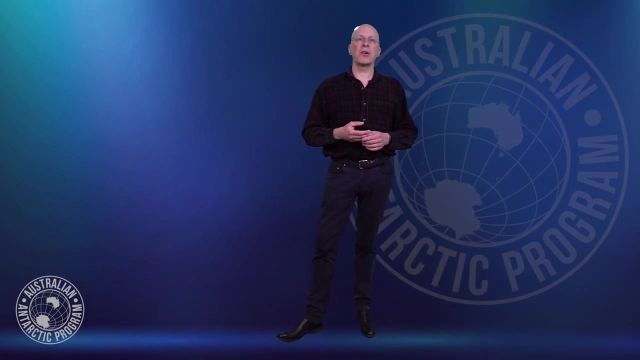 oceans as a whole plays a really important role, buffering our climate system. In total, the oceans of the planet have soaked up something like 30% of the CO2 we've ever emitted and more than 90% of the heat. What happens to this buffering as we go forward is a really critical question if we're 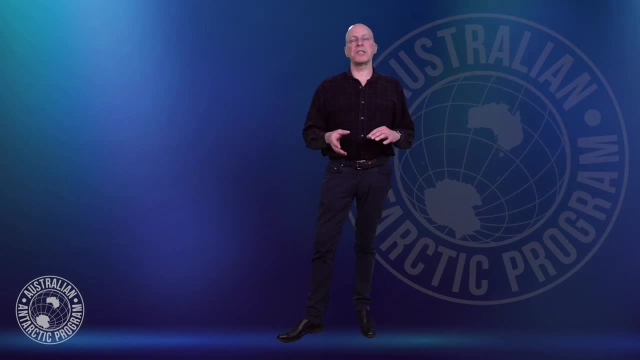 going to predict the future and we're part of international efforts to monitor the Southern Ocean and measure the currents and the properties and look for signs of change and ensure that we understand what's going on. So the final part of the climate machinery that we look at is the 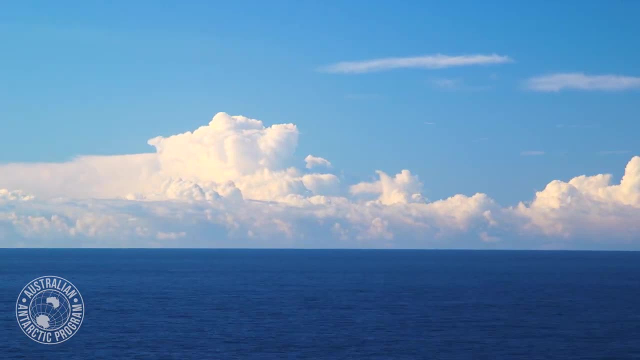 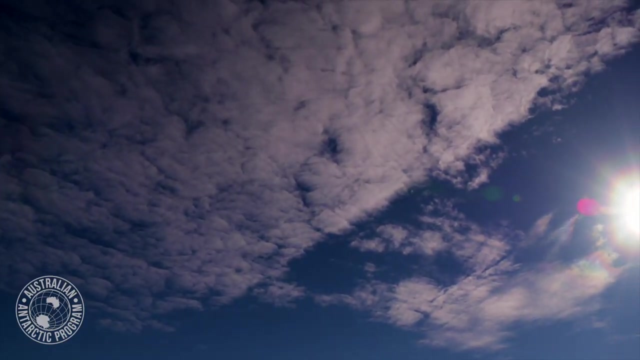 atmosphere over Antarctica and the Southern Ocean. The atmosphere, like the ocean, is a fluid component, moving heat and water around the planet, connecting the tropics to Antarctica and connecting Antarctica back to mid-latitudes and Australia in particular, And the Antarctic atmosphere has changed as a result. 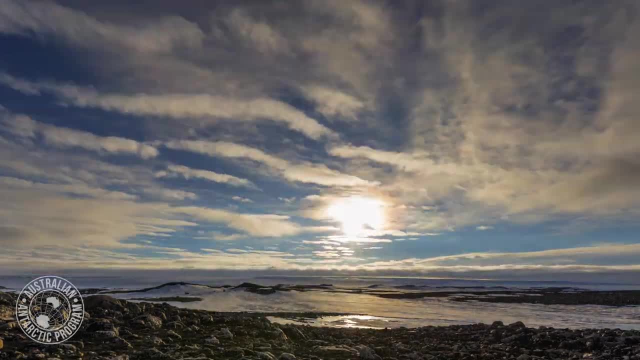 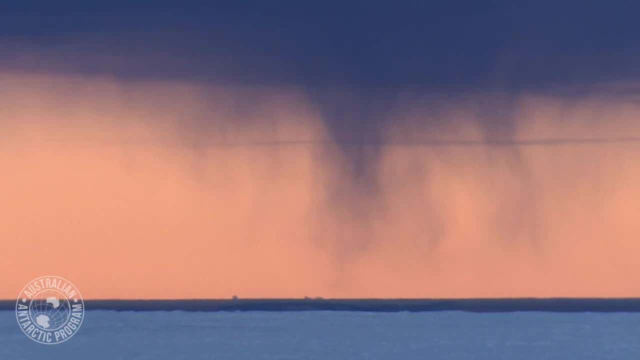 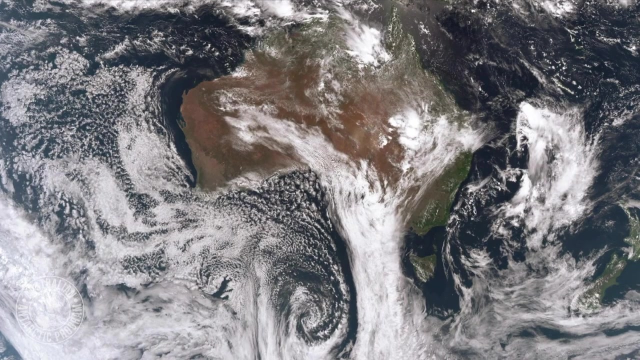 of human activity, Mostly ozone depletion, the ozone hole, but also CO2.. These things have changed the temperature structure of the atmosphere above Antarctica, cooling the stratosphere and above and actually strengthening the winds that circulate around Antarctica, These westerly winds that circulate. 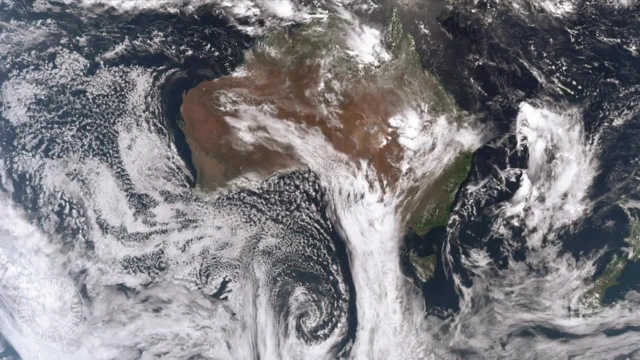 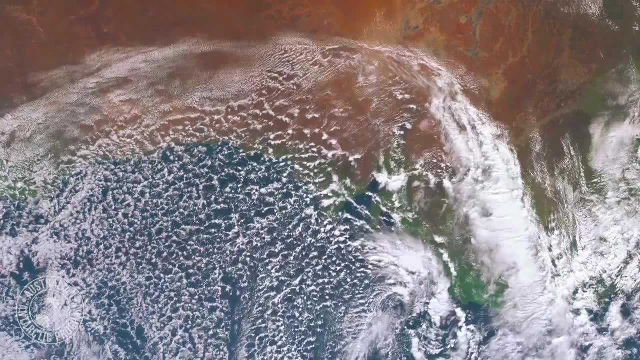 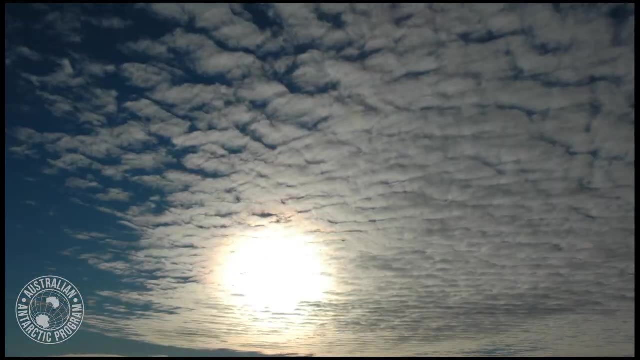 around the Southern Ocean have not only strengthened, but they've shrunk towards the pole, southward, taking with them some of the rain bearing fronts that actually intersect Southern Australia and the Antarctic. We're also concerned, when we talk of the atmosphere, about the clouds in the Southern Ocean, which play a really important role. 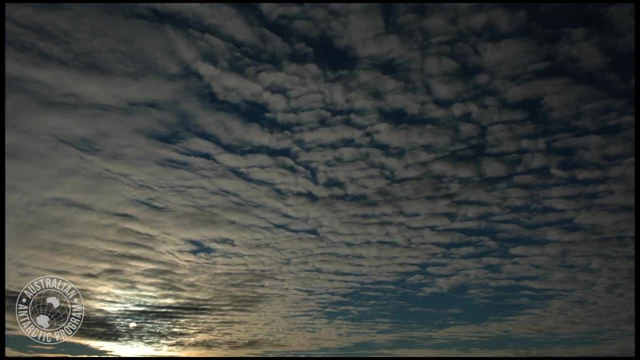 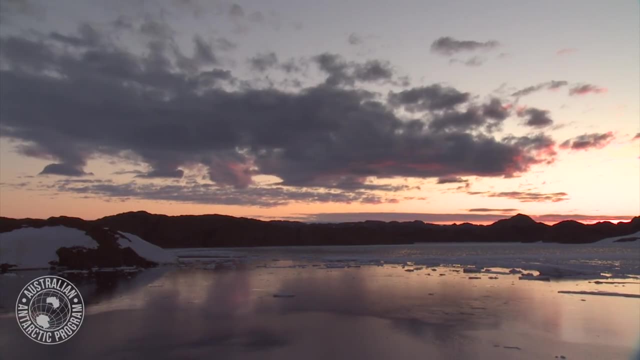 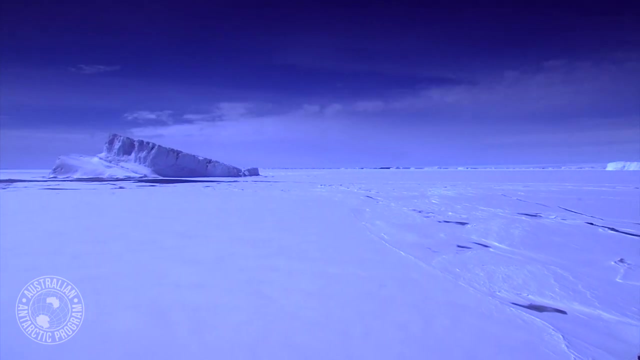 reflecting light back to space and controlling the amount of heat which actually reaches the ocean below That reflectivity is critically dependent on the mix between ice and super cooled water in the clouds, and scientists are carefully modelling and understanding that mix so that we can do a better job of predicting weather and climate into the future. 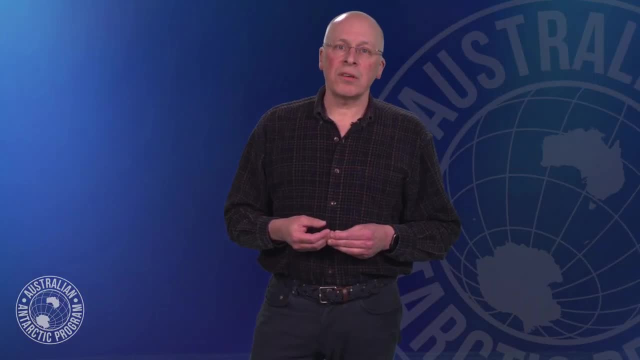 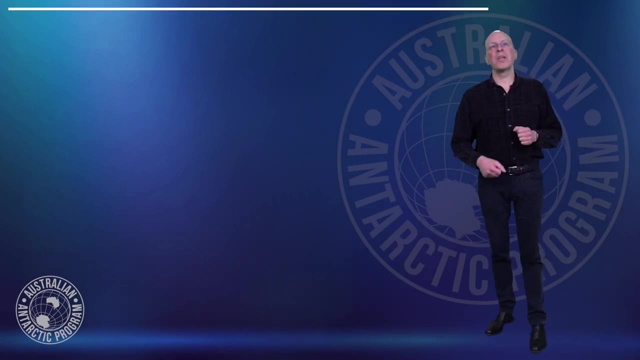 As we look to the future, we think also of the deeper time in the past, And so, if we look at that three kilometre time machine I referred to earlier, we can drill ice cores that go all the way to the bottom of the ice sheet. 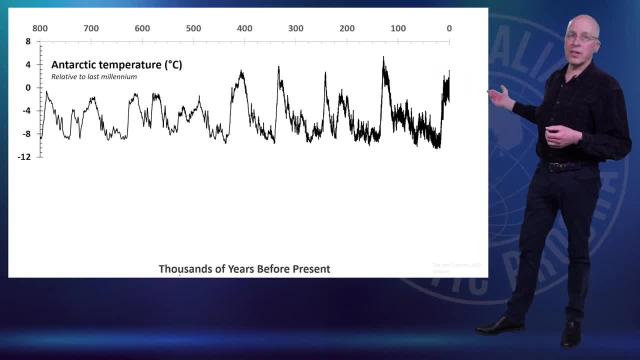 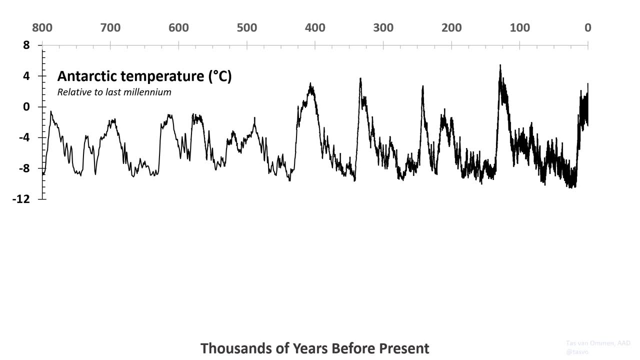 Presently the longest of these is a core that goes back 800,000 years. This 800,000 year ice core shows us in detail how the climate's waxed and waned over that period. We've seen warm periods like the present. 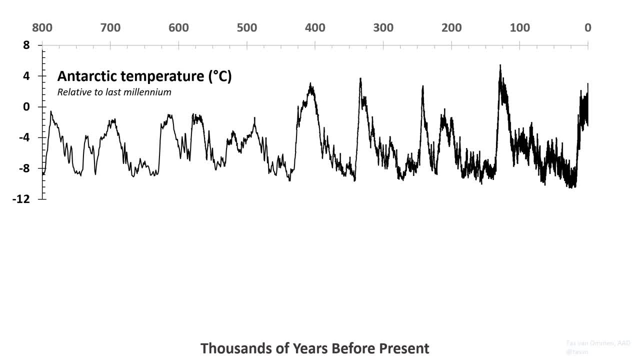 it's been disbursed with cold periods where there were ice sheets over North America and northern Europe. This pulsing we see in the chemical signatures from the ice core shows the climate over that time period. But we also see from the ice core something else, Trapped between the snowflakes as it gets buried. 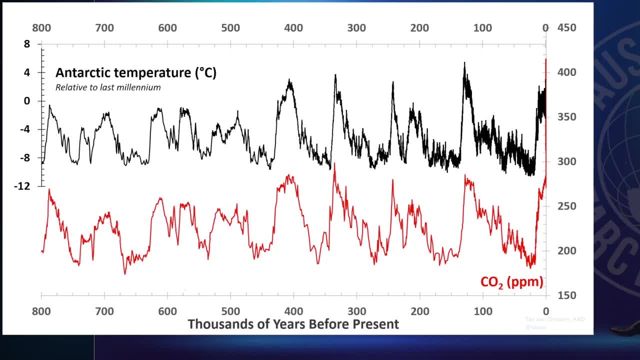 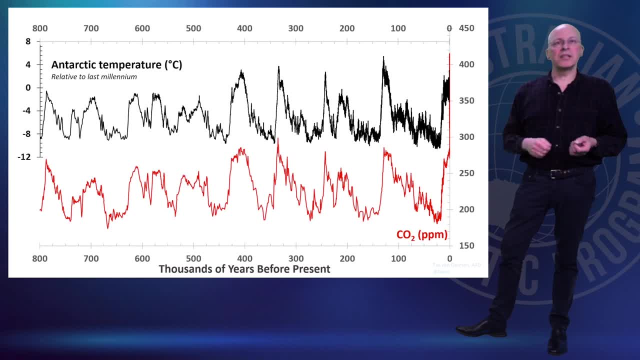 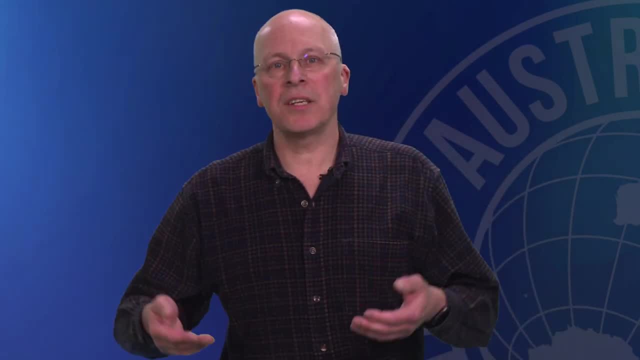 we get bubbles of past atmosphere and when we crack open those bubbles we can see CO2 levels. What we see is CO2 over those 800,000 years looks remarkably like the temperature, amazingly so. This shows us that temperature and CO2 on the planet are tightly coupled in the natural 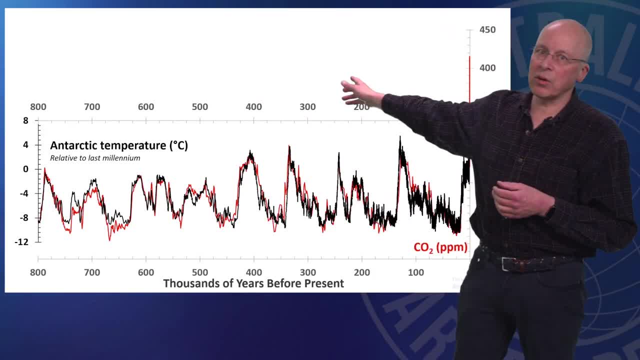 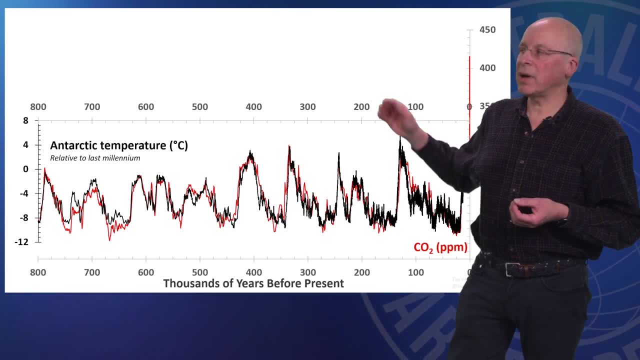 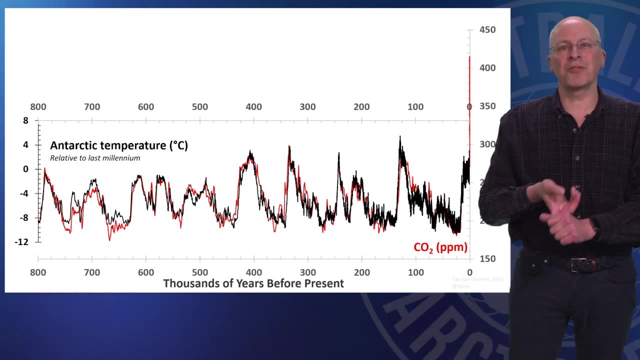 system. That is until we come to the recent period. If you look on the far right, you can see how the CO2 has increased its industrialisation to levels well above anything seen in the 800,000 year record, Even before we turn to our well understood physics of greenhouse gases and our climate. 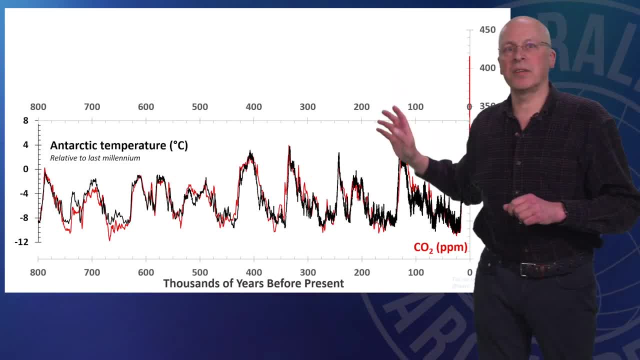 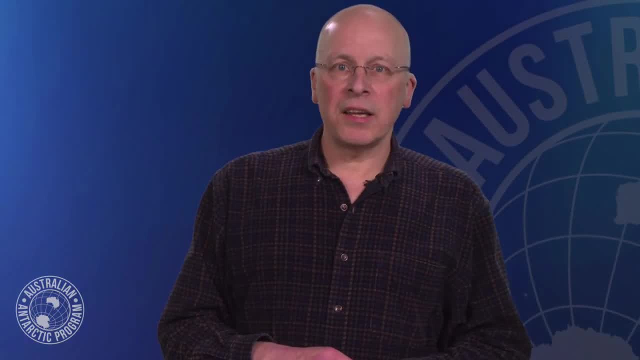 models. the ice is telling us that things are going to be different in the future than they were in the past. You will have heard in what I've been saying a recurring theme- that, while we understand Antarctica and the Southern Ocean much better than we did and we know a lot more about 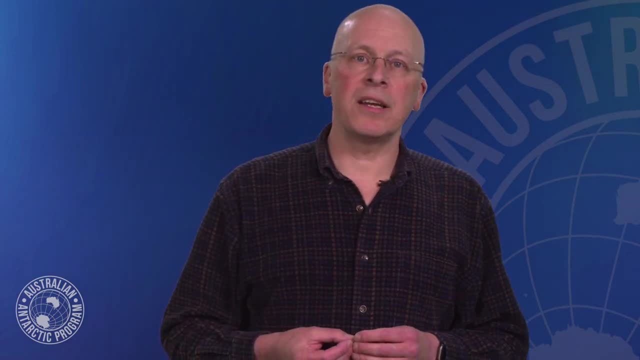 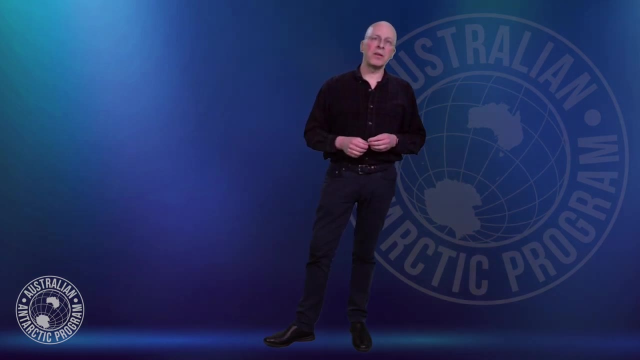 the climate system. there are still really important gaps in our understanding, Gaps that matter to our ability to project what's going to happen in the future. And if we look to the future, I'm reminded of the words of former White House advisor on climate, John Holdren, who 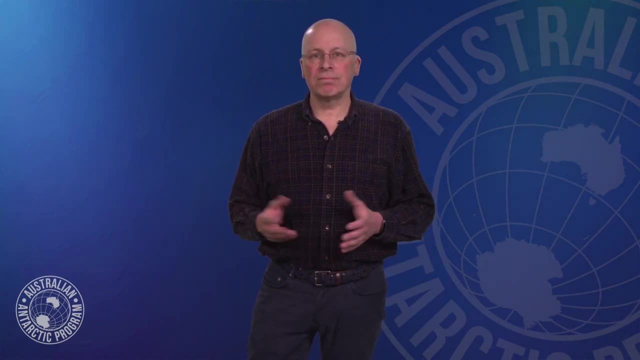 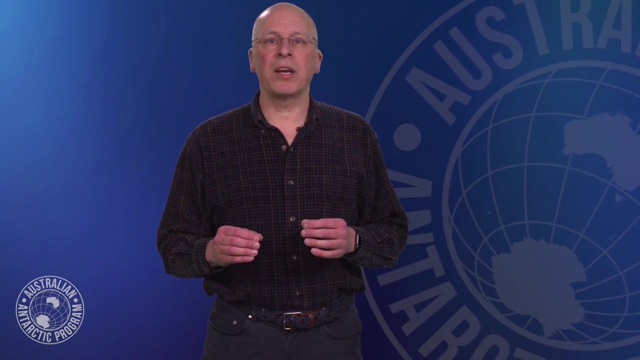 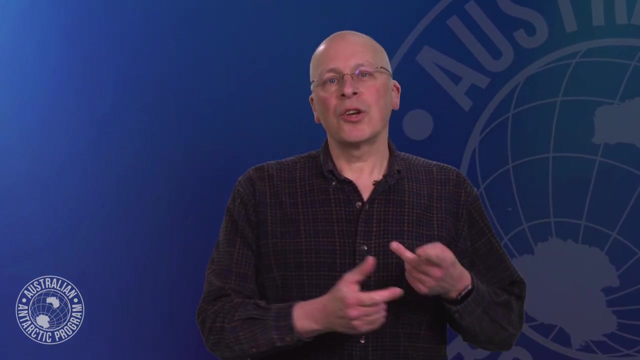 said, all we have is adaptation, mitigation and suffering. As a scientist, my hope is that we can use our understanding to chart a pathway to a resilient future. Knowledge is power. Knowledge will tell us what we absolutely need to avoid, Knowledge will guide our adaptation and knowledge will help reduce suffering. 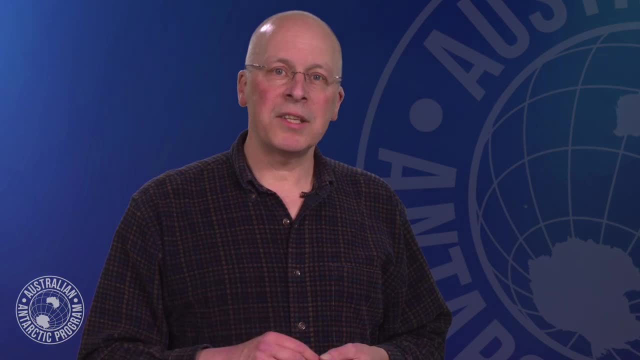 And thinking back to that question, That cold night on the Antarctic plateau, there's the answer to my question. That's why I do what I do.